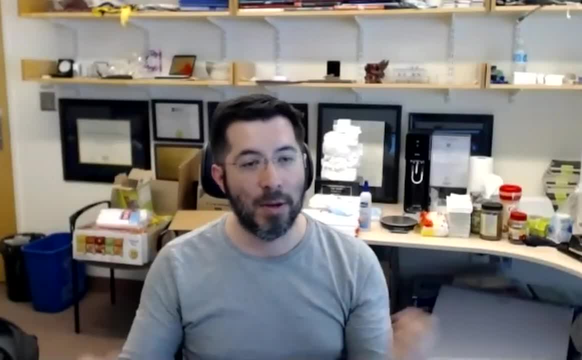 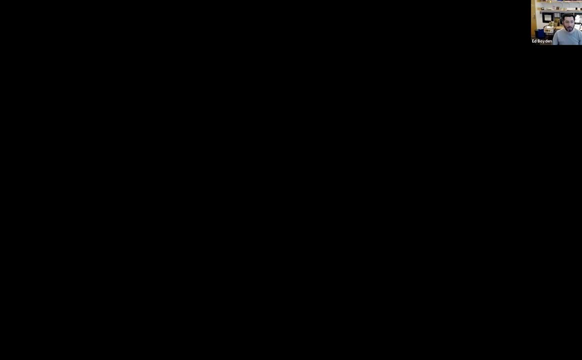 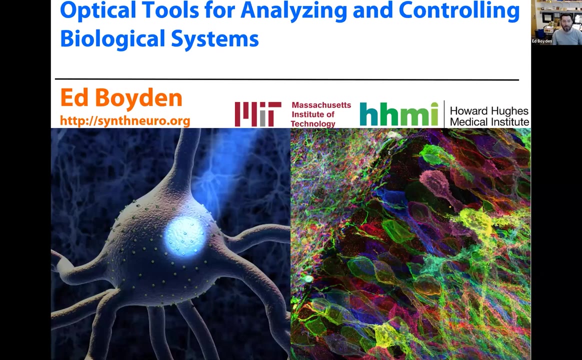 build tools that enable very detailed mapping, imaging and control of biological systems with a focus on the brain. Let me share my screen here. Okay, Is that showing up? Oh, there's a Zoom window at the bottom. How can I make it not cover the talk? Okay, We see it. well, so far, Ed. 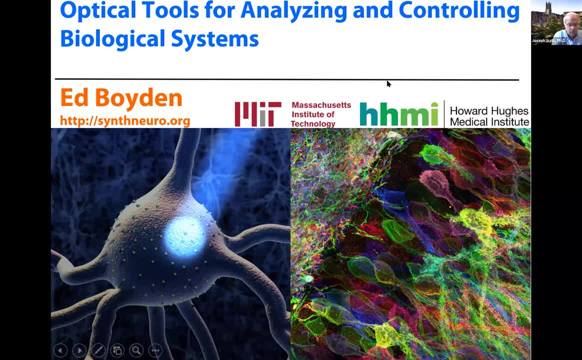 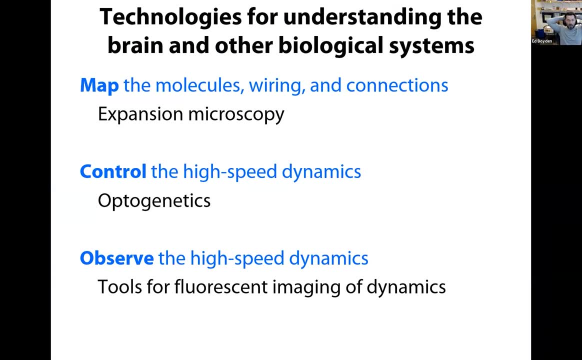 Okay, great. So our group really thinks a lot about the spatial and temporal scales over which biological systems like the brain operate. Biomolecules, gene products and so forth are, after all, nanoscale things, But organ systems like the brain are enormous. 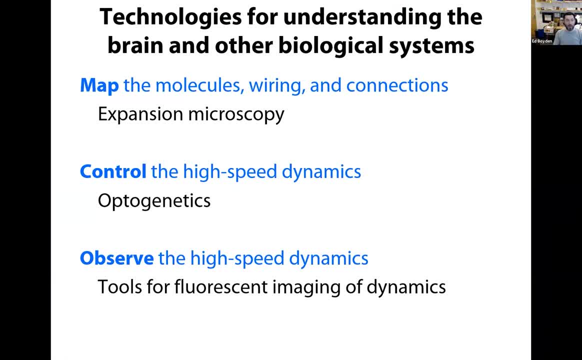 right. How can you see nanoscale things across large 3D expanses? And the time domain is no less daunting. High speed biological signals in the brain can last a millisecond or less, But brain aging, memory formation, the changes of brain states, can take days. 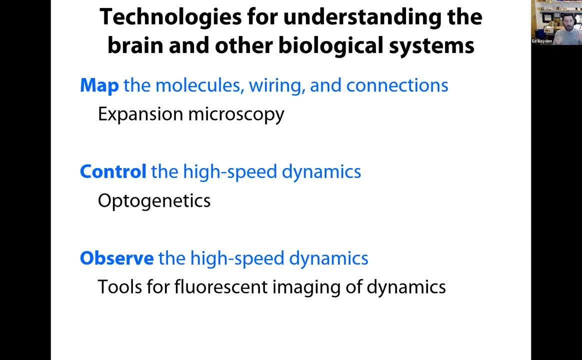 months, years and even years, And so we're trying to build a system that allows us to do that. So I sometimes only half-jokingly say that our goal as a group is to figure out how to help biologists cross space and time, And these are not unique problems to the brain, If you. 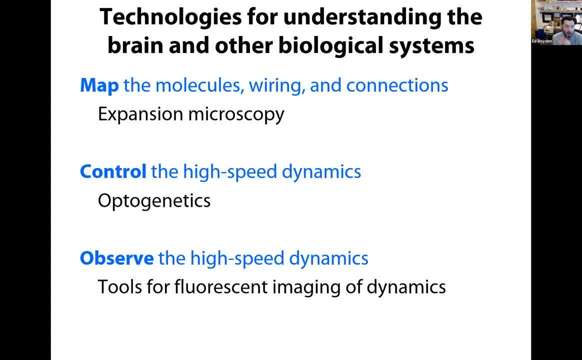 study the immune system, or aging or the spread of a cancer. we also deal with vastly different spatial and temporal scales. So today I'll tell you three short stories, one about space and two about time, with the hope of explaining some of the technologies we've built that we hope can help. 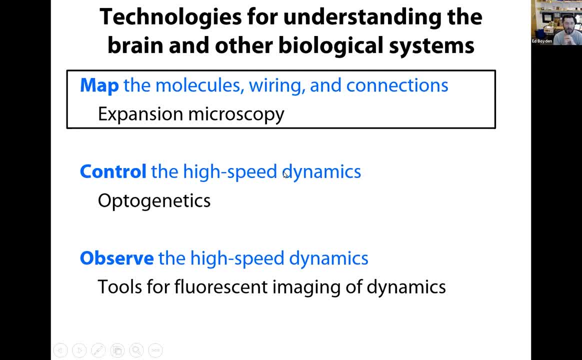 people cross these different scales. Let's start with expansion microscopy, which is a way to help do nanoscale imaging of extended 3D objects. So, of course, many pioneering microscope designers and physicists and chemists have developed fantastic nanoimaging methods, super-resolution microscopes, for example. 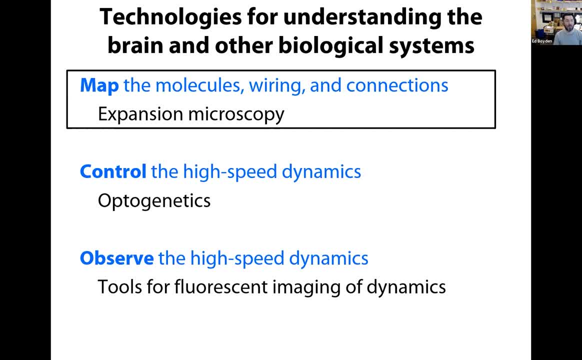 other forms of physical interfacing, such as electron microscopes, cryo-EM and so forth, But all these methods struggle to image large 3D objects like a brain circuit, And they also, as a result, can require extensive equipment and or skills. 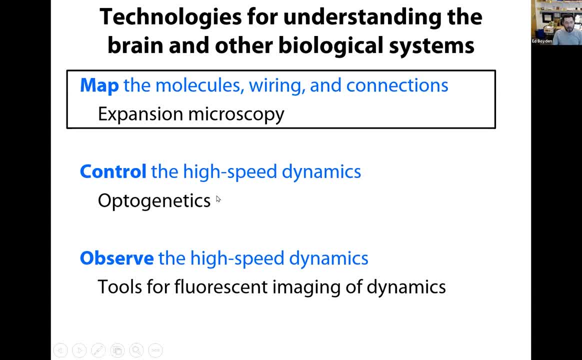 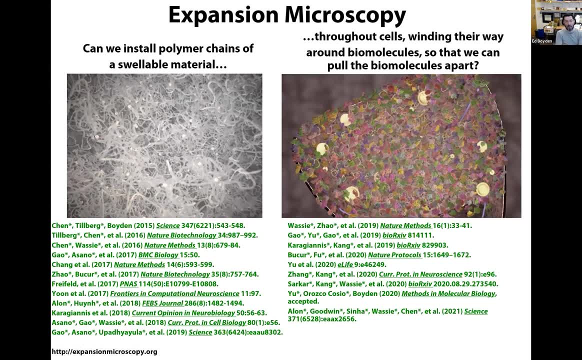 So our group, we often try to think about: you know, can we do the opposite of what people have been doing? And so we started thinking: what if we tried to physically magnify a biological specimen? So of course this is not a living thing anymore, but suppose you could chemically synthesize a dense. 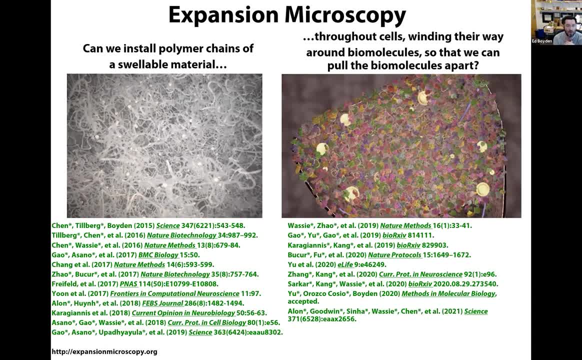 spiderweb-like mesh of swallowable polymer throughout a preserved biological specimen. Weave those threads of swallowable polymer inside cells and outside cells in between biomolecules and then around biomolecules. If you anchor key biomolecules to the polymer, soften the specimen through. 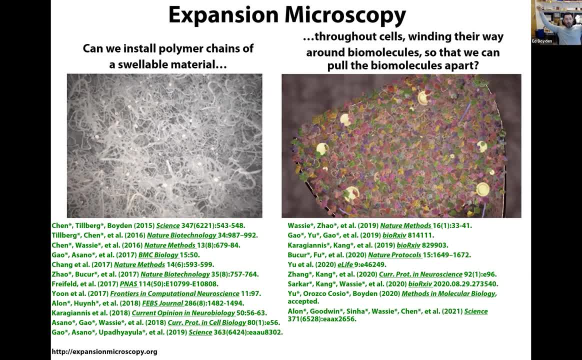 chemical treatment and add water, the swallowable polymer will grow, but because of the little handles that we use to bind the biomolecules to the polymer, the biomolecules will be pulled apart. In other words, we could physically magnify a biological specimen, which we call expansion microscopy. 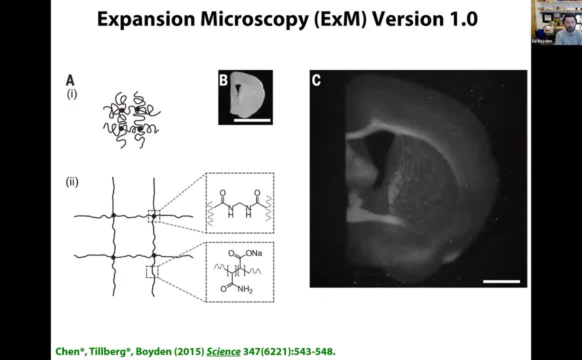 So we first announced this discovery that we could evenly expand a biological specimen in 2015,, led by two then graduate students in my group, Pei Chen and Paul Tilburg. Panel B is a small piece of the mouse brain before we expand it. Panel C, it's about 100 times bigger. 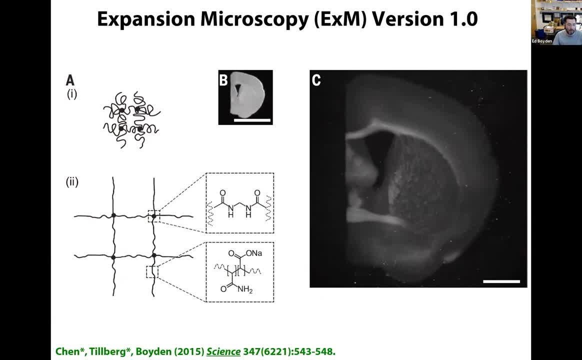 We've created a dense, spiderweb-like mesh of sodium polyacrylate, maybe better known as the active ingredient in baby diapers, and we have physically blown it up by about 100 fold in volume, four and a half fold in each direction. 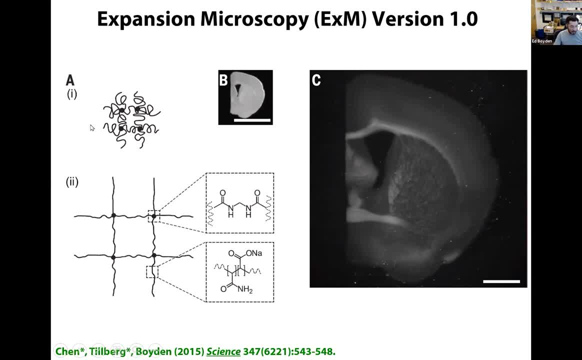 The polymer threads start out very dense, just a few nanometers apart, comparable to the size of a biomolecule, and then we can end up with something like the cartoon in the lower left, where the polymer threads are pulled apart from each other. 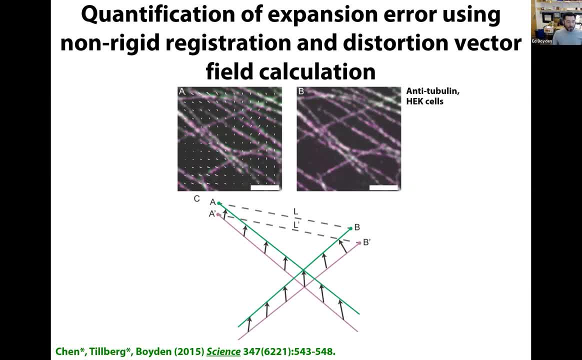 First question I always get: is it precise? Well, it's pretty good. We get distortions of a few percent over a typical microscope's field of view and it turns out for the vast majority of biological questions that's what we want: the relative organization of biomolecules. 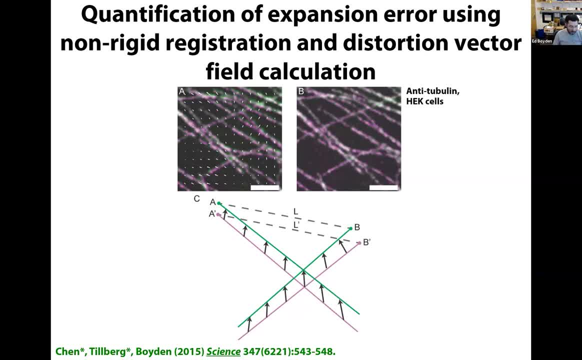 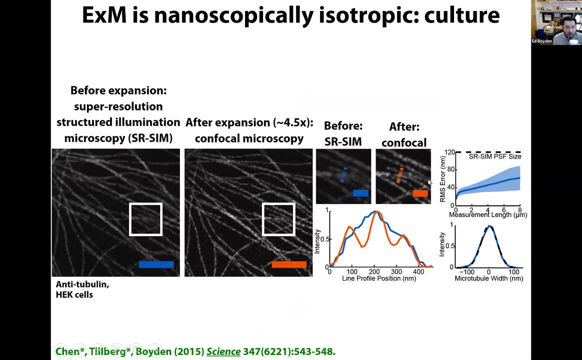 We've done lots of pre versus post comparisons, like shown on this slide, to measure the amount of distortion that is incurred. We can also measure the resolution. so on an expand by four and a half fold on a 300 nanometer resolution lens, the typical microscope lens- would. 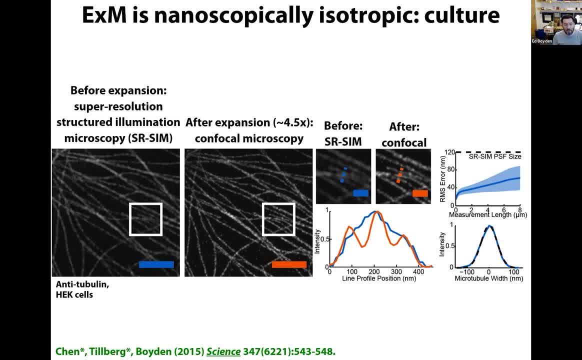 electron microscopy and we get a resolution of around 65 nanometers, which is what we expected. Now, you might remember that polymer spacing is really tiny, just a couple nanometers. If we expand more, can we get better resolution? And, as I'll show you, the answer is yes. 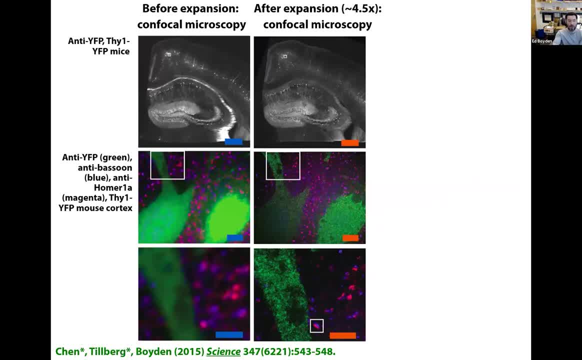 but even with four and a half fold expansion, there's a lot of things you can do that are difficult and sometimes even impossible to do with earlier techniques. So here on the left-hand side is the Phi-1, YFP, mouse cortex and hippocampus. Each white square is zoomed into the region below. 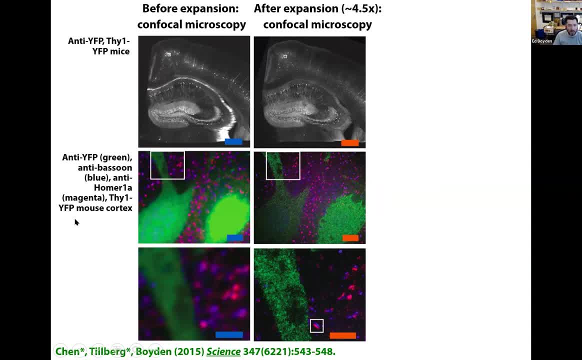 The color code is shown on the left again. fluorescent antibodies against different proteins. This is taken on a conventional confocal microscope And on the right is the same specimen, same fields of view. but after we've expanded You can see much more detail And in 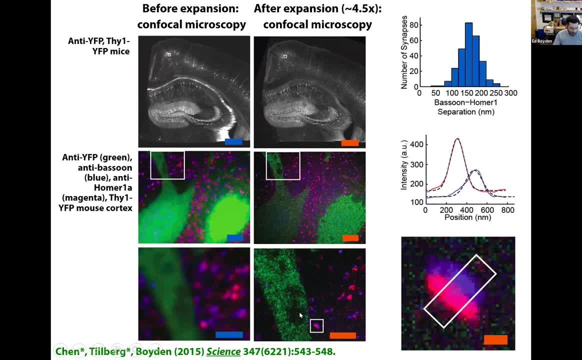 fact, the purplish blobs on the left are cleanly resolvable on the right in terms of these blue and magenta protein densities. Blue is the presynaptic protein, bassoon Magenta is the post-synaptic protein HOMER1a. And the distance. 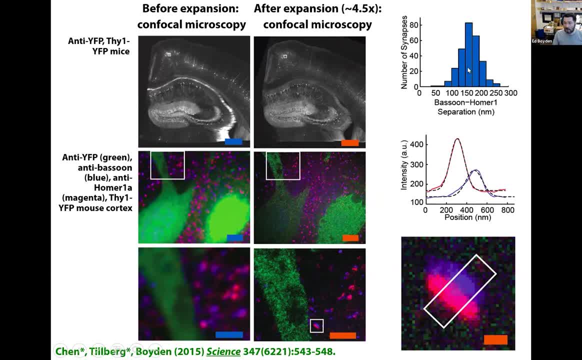 between these protein centroids is the same distance that Catherine Duloc and Zhao Yizhuang measured many years ago with storm microscopy, And now we can make this measurement on a conventional confocal microscope. This is some work that we did with Eric Betzig's group expanding. 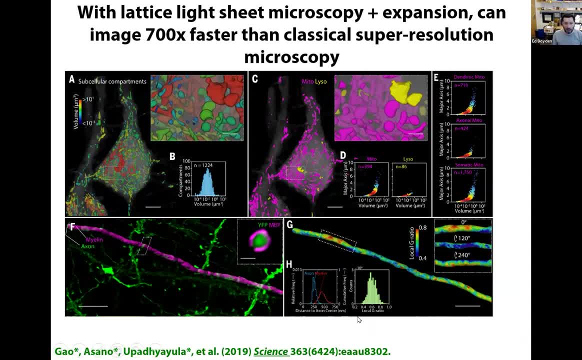 and then taking advantage of the transparency of an expanded specimen by using light-sheet microscopy to go at blazingly fast speeds. In the upper right we can look at mitochondrial and lysosomal proteins. At the bottom, you can see, here we're looking at myelin. This is work triply spearheaded by Ray Gao. 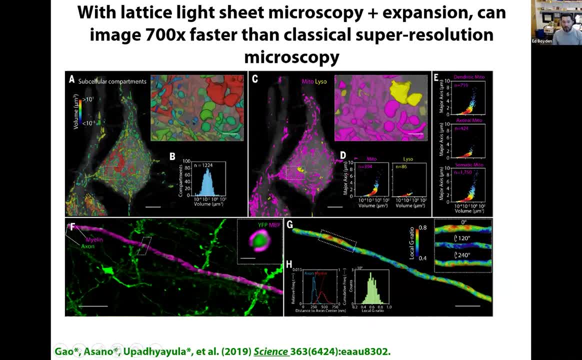 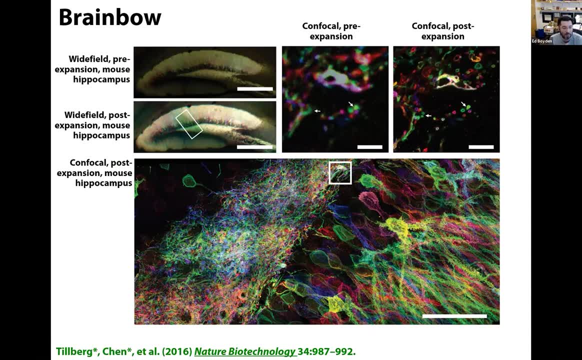 Zhou Asano and Gokul Apariula working across our two groups. You can express artificial proteins such as fluorescent proteins engineered from jellyfish and coral. Here we are doing brainbow, where we express combinations of fluorescent proteins using viruses in the brain. So different neurons exhibit different physical 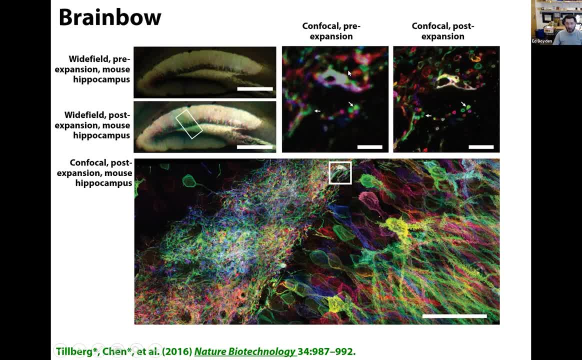 color codes And, as you can see at the top, quickly, of course we hit the resolution limit of the microscope, But if we expand and then image, we can cleanly resolve in the upper right-hand corner individual axons. This happens to be in the pilus of the mouse, hippocampus. 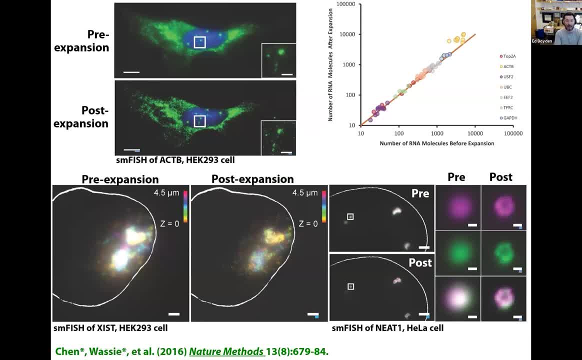 So far, what I've showed you is protein visualization, but we can visualize nucleic acids as well. Oz Wasi joined the team and co-led a project along with Fei to expand protein and RNAs away from each other, And then we can do post-expansion in-situ hybridization against the. 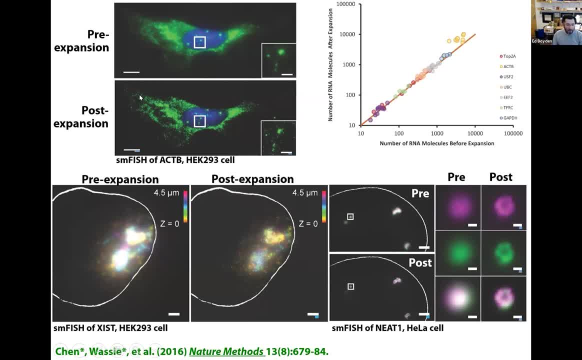 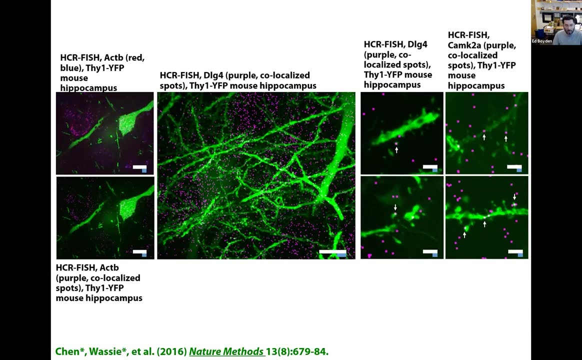 RNA. Here you can see in the upper left, beta-actin in the lower left exist and the lower right need one, And we can do these in cell culture as shown in this slide. But we can also do post-expansion in-situ hybridization against RNAs in intact brain circuitry. So here we are looking. 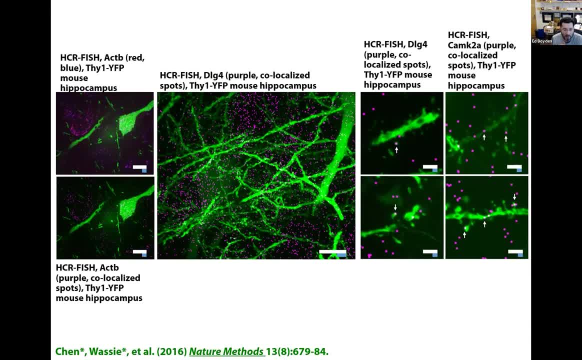 at a specimen of brain where we've anchored and expanded proteins- You can see YFP here, for example- And also RNA. And then the magenta dots are individual RNAs. So we can image with nanoscale precision the location and identity of individual expressed RNAs throughout brain circuits. 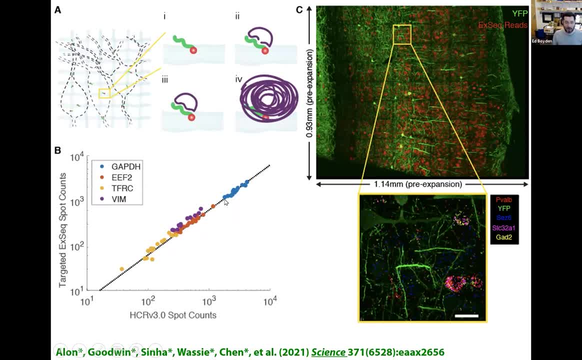 We can do multiplex analysis of RNAs. So many pioneering scientists have developed ways of using libraries of hybridization probes against RNAs to look at dozens, even hundreds, in a single sample, In work that was quintuply spearheaded by Shahar Alon Dan Goodwin. 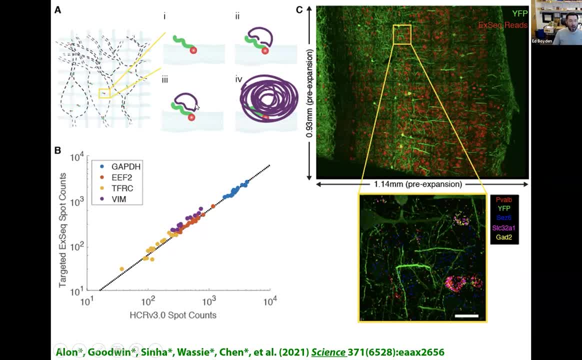 Anu Sinha Azwasi and Fei Chen. we brought in hybridization probes against RNAs and then would sequence little barcodes on the other side of these so-called padlock probes- so-called because of their shape, And the barcode is not shown here, but we can sequence it. And when you sequence the 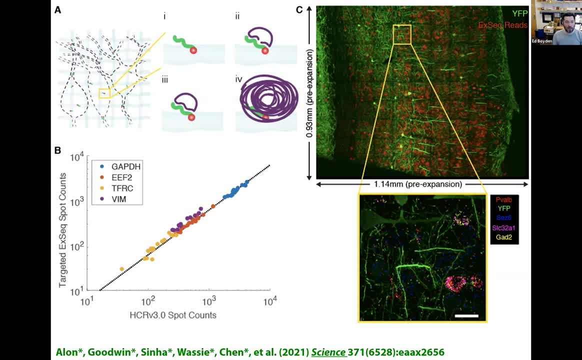 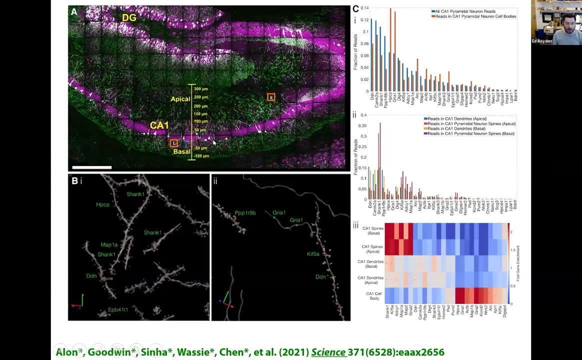 nucleic acid. you're just copying it. As you copy it, you're adding fluorescent nucleotides, And so we can do that in intact brain specimens. Here's just one example here where you can see that this is a cell that's filled with YFP, And we can look at individual messenger RNAs. 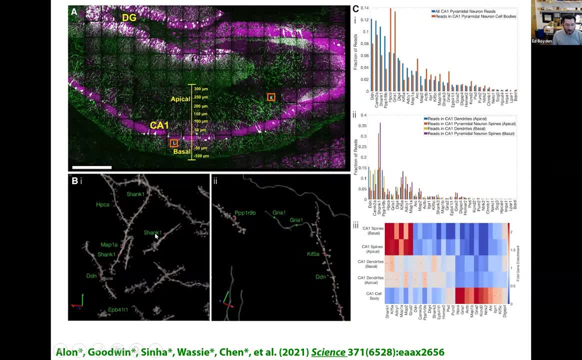 taking a cue from Erin Schumann's wonderful surveys of dendritic RNAs, We synthesized about a couple dozen probe sets against RNAs identified by her group and other groups, And we're able to pinpoint with nanoscale precision individual RNAs from a library of these several dozen. 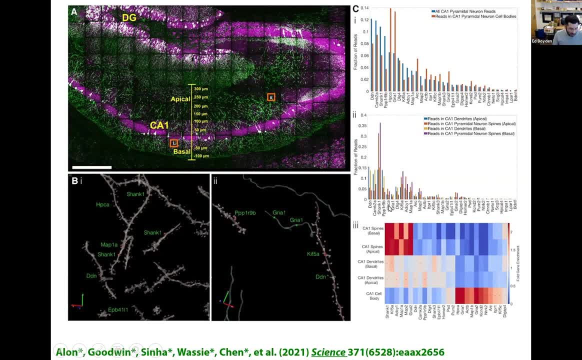 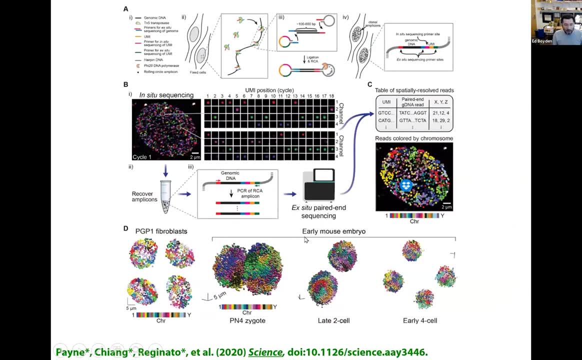 messenger RNAs And we can derive interesting patterns, shown in the lower right, about how these RNAs are distributed throughout different parts of brain cells. As a bit of a side note, this doesn't involve expansion, not yet anyway, but we saw an. 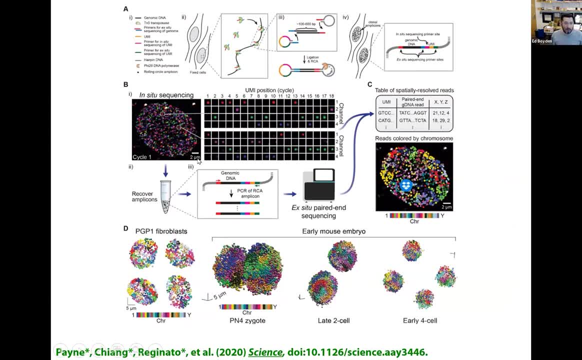 opportunity to use this kind of in-situ sequencing strategy to look at the genome as well, And so, in a collaboration with Jason Van Roster and Fei Chen's groups led by Andrew Payne, Zach Chang and Paul Reginato- working across the two groups- three groups, excuse me- we showed that we could. 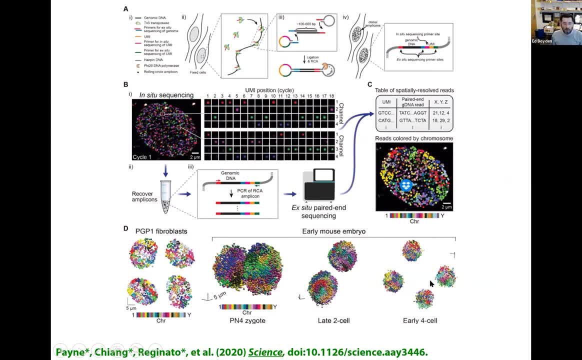 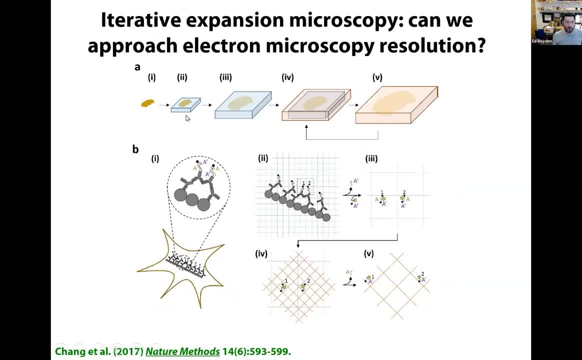 the genome. We asked: could we expand the genome? We asked, could we expand the genome More than fourfold? And when JB Chang was a postdoc in the group, we plimarized and expanded a piece of brain, as shown in the cartoon in the upper left, from a second polymer in the space opened up by 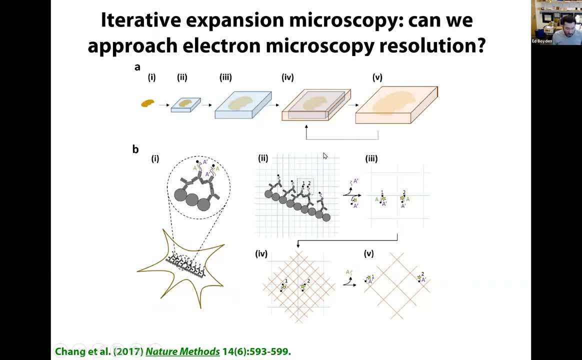 the first expansion and expanded it again. So fourfold expansion times, fourfold expansion should give you about 15, 16 fold expansion. Now, this original version, which we published in 2017, was a little bit punky, And so, since then, Diblina Sarkar, Jin-Yun Kang and Ozwasi. 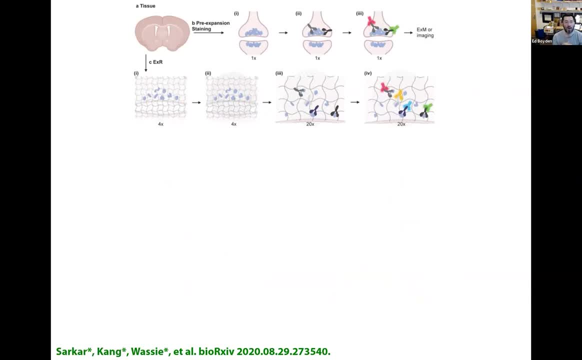 with great help from Margaret Schroeder and Christina Kipco and M Becomenari have developed an important version of this as well. we developed a way of doing the double expansion process using all off-the-shelf chemicals And we noted this has an interesting possible bonus In the cartoon. 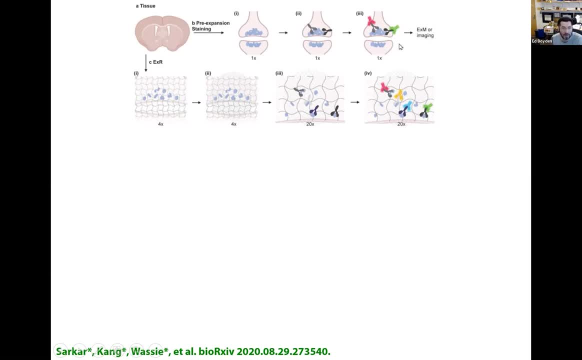 at the top, you can see the green and red antibodies binding to proteins on the outside of a complex. But can you get to the inside of a protein complex? After all, most proteins have the opportunity to participate in 3D architectures within cells. Well, if you pull. 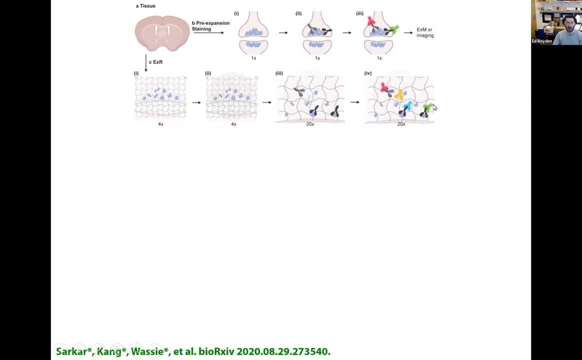 proteins apart from each other. maybe, as shown in the cartoon in the lower right now, the blue and the yellow antibodies can get inside and access epitopes that are otherwise hidden. We decided to see if we could look at synapses, which, of course, are very dense. 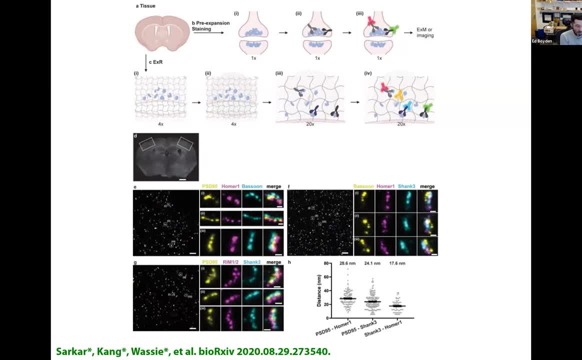 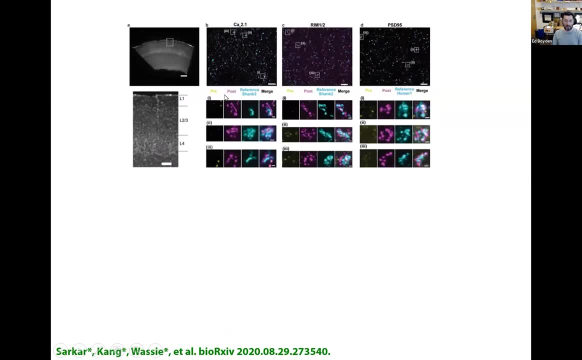 and compactly arranged agglomerations of proteins to see if we could actually resolve and identify previously invisible proteins. Well, here in panels B, C and D you can see yellow pre-expansion staining and three red London-based proteins, As shown, indicate the presence of pre-expansion staining on the blue and yellow antibodies. 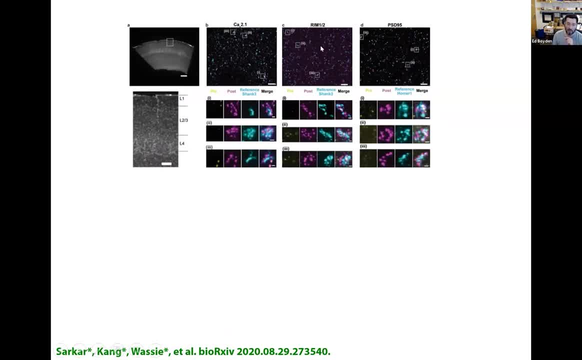 purple post-expansion staining of a calcium channel subunit, a presynaptic protein and a post-synaptic protein. And yes, there's a lot more purple than there is yellow. So decrowding the proteins from each other helps get access to the inside of these complexes. Not all proteins are. 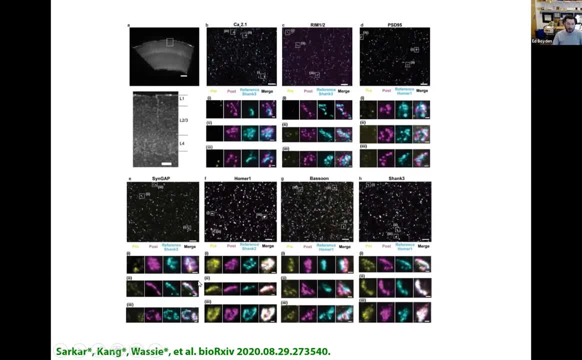 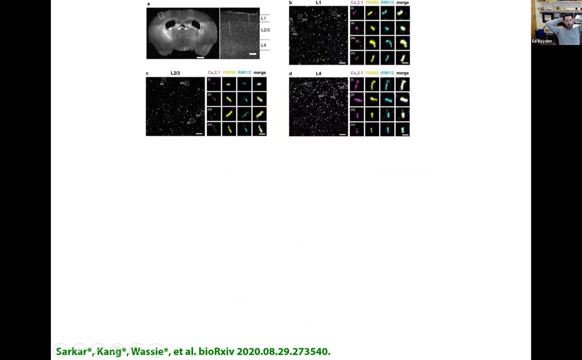 so crowded. F, G and H show three proteins that have comparable yellow and purple. So we started wondering if we can see proteins now by decrowding them and enabling them to be better stained. are there things now that we can reveal that are difficult or impossible to see using other? 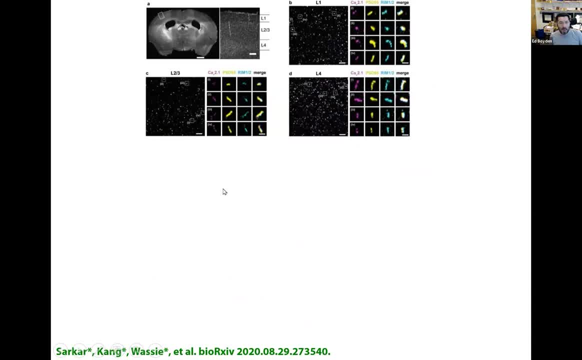 techniques, And so, working with Tom Blanke's group, we decided to look at these nanocollabs, coordinated pre- and post-synaptic proteins, to try to see if we could see organization of, let's say, that new calcium channel that we just pointed out and post-synaptic proteins. 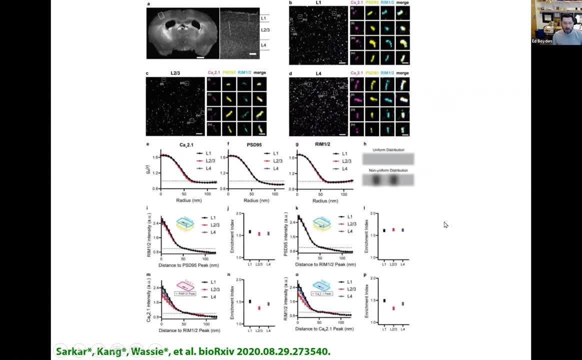 And, to make a long story short, we did see detailed coordination of pre- and post-synaptic proteins. They were not uniformly distributed, but instead were coordinated across the synaptic cleft, And so this might help with the precision of nanocollabs, And so we decided to look at these nanocollabs coordinated: pre- and post-synaptic. 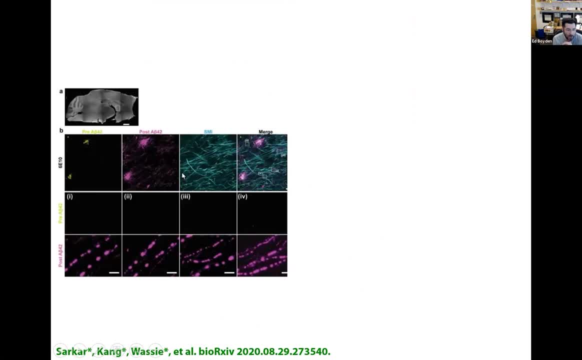 neurotransmission. Working with Li Wei-Sai's group, we looked at amyloid plaques, also extremely densely packed things. These are in 5XFAD model. mice Yellow is pre-expansion of an antibody against A-beta-42.. Magenta is the same specimen, same antibody after expansion, And I hope you. 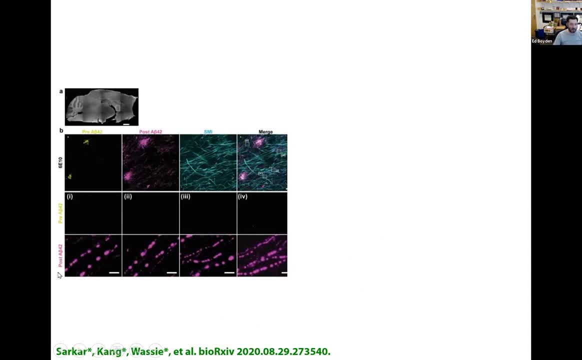 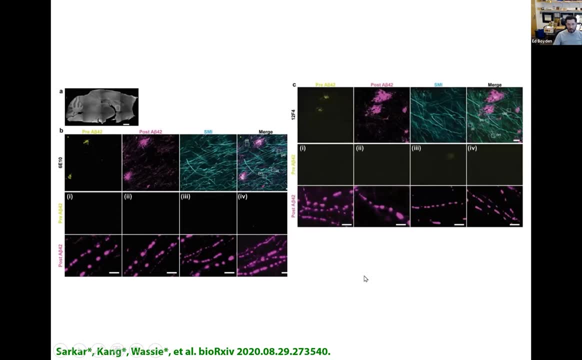 can see, the purple images have a lot more detail than the yellow. In fact we even saw these amyloid dots, almost periodic structures, at the bottom here, And this held for two different A-beta-42 antibodies, and we did not see them in wild-type mice. So we're very excited now that expansion. 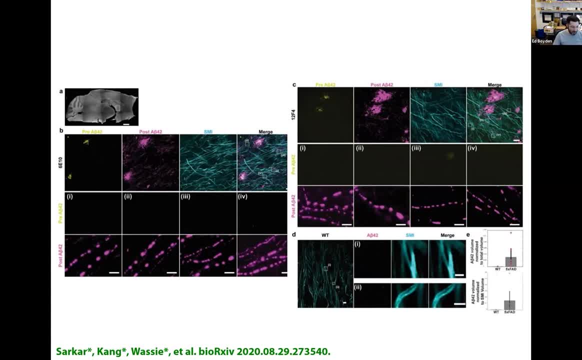 microscopy not only allows us to democratize nanoimaging- now we can do nanoimaging on regular old microscopes- but it might also, by decrowding molecules from each other, enable interesting reactions, like the sequencing methods that I mentioned earlier, or allow for better staining. 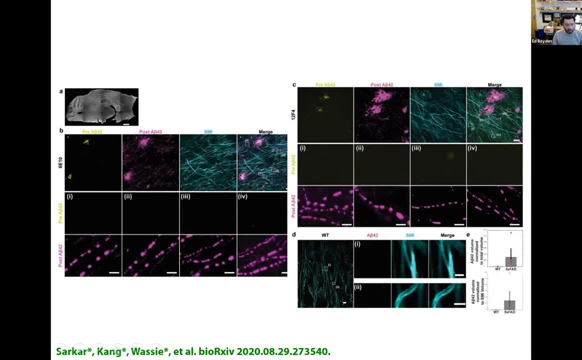 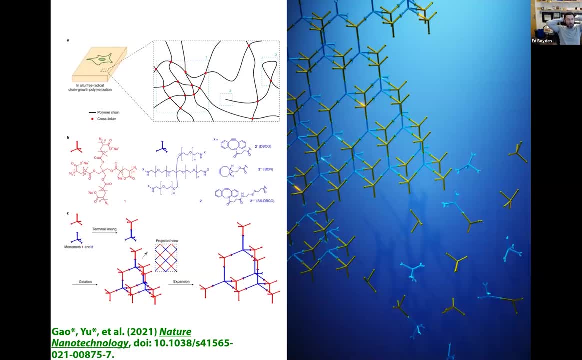 and labeling of densely packed molecules in complexes. How precisely can we expand? Well, at some point we're going to have to figure out how to do that, And so we're going to have to hit the limit of the resolution of the polymer itself, And it turns out the polymer, of course. 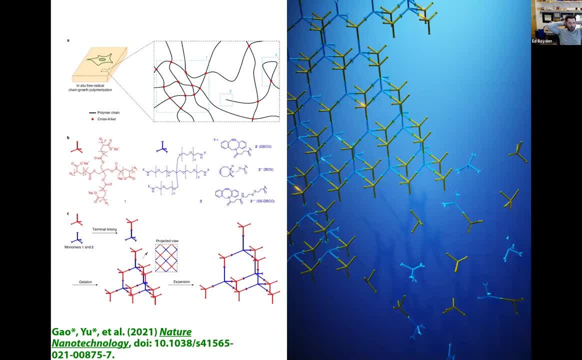 has a lot of inhomogeneities. These are classical free radical synthesized polymers, And so, Ray Gao and JU and our group, we decided to investigate whether we could use these so-called diamond lattice polymers to get much more even expansion. These are known in the field of polymer chemistry. 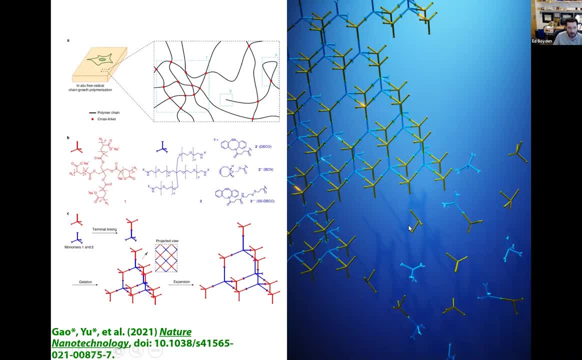 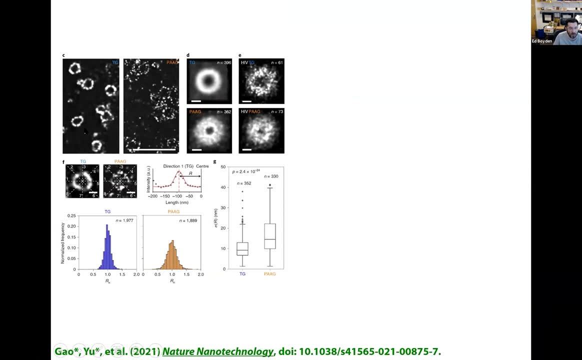 to yield almost perfect, defect-free lattices. They're made out of these tetrahedral monomers such as shown in the cartoon at the right. Using viruses as sort of a natural scale bar, we showed that this so-called tetragel 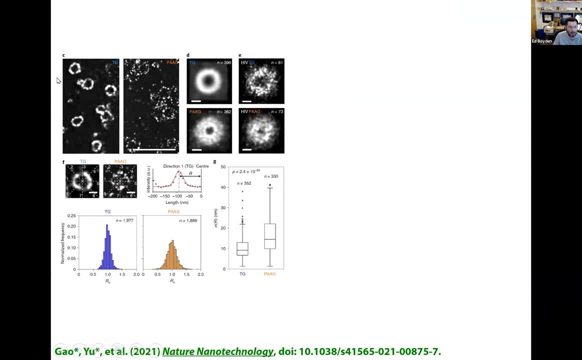 as shown in the upper left, could result in very nice, evenly expanded viral shapes. The older free radical gel. as shown in the right-hand panel of C, you can still see the rough circularity of the virus, but the shape is not as well preserved, And so in panel G, 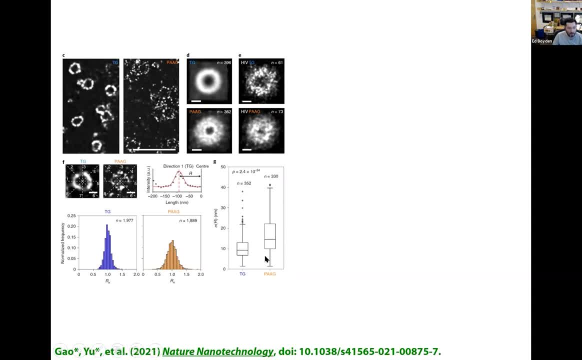 we saw that the resolution indeed improved. The accuracy of the expansion improved from 15 to 20 nanometers or so. So we're excited that this might be the first ability to get down to single nanometer resolution imaging- on an ordinary microscope for that matter. 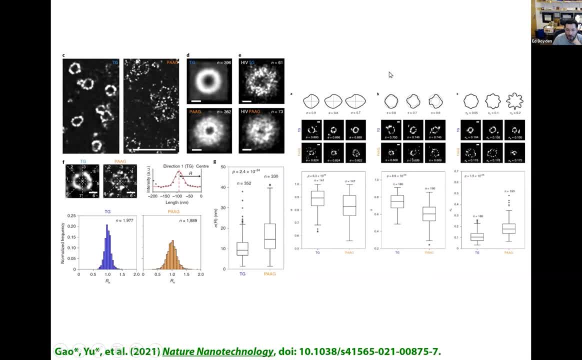 So this is some examples here on the right of shapes, of different viruses, excuse me of herpes simplex virus. I forgot to mention the virus. We're evaluating ellipticity and sphericity and other measures of shape, And indeed the shapes are better preserved with. 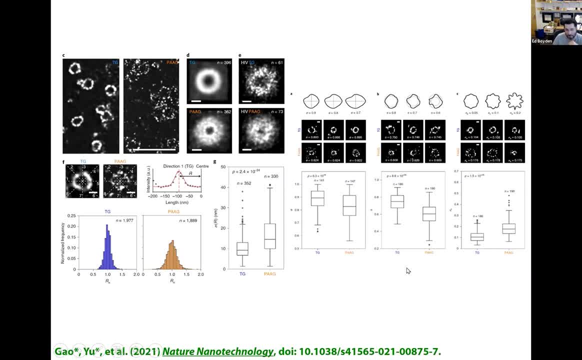 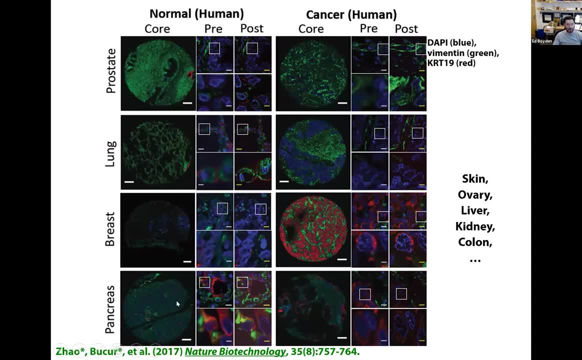 this tetrahedral hydrogel Than with the original. Of course, you can apply this to human tissues. This is work done by Yangxin Zhao and Octavia Bucure, working between our group and many pathology groups like Astrid Weins, Andy Beck. 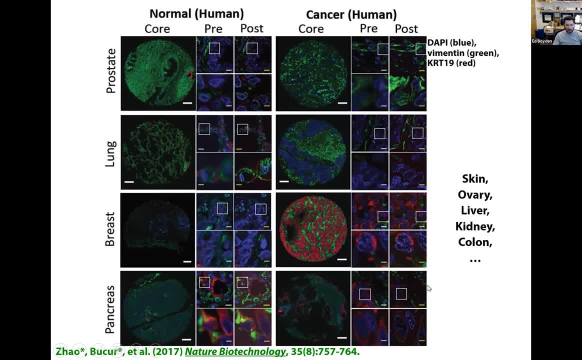 and others On the left are normal and on the right are cancer-containing specimens from human patients And basically we have a lot of off-the-shelf, easy-to-use protocols. So let me summarize by showing a slide. that's really not meant to be read, but it's meant to. 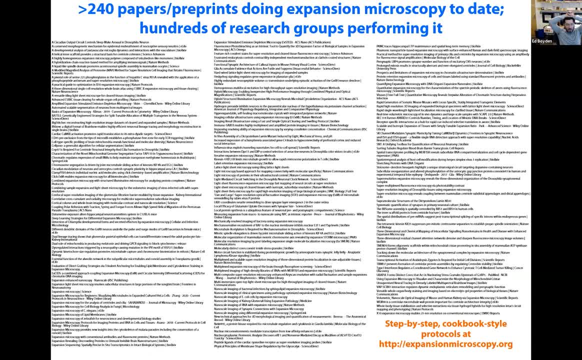 really convey that expansion of microscopy is very important. So this is an example of an experiment that we're doing. This is an experiment that we're doing. It's going to be spreading very quickly. Over 240 experimental papers and preprints have come out. These aren't like commentary pieces. These are actual experiments, people. 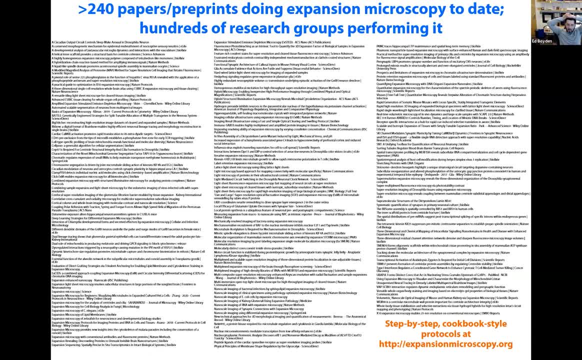 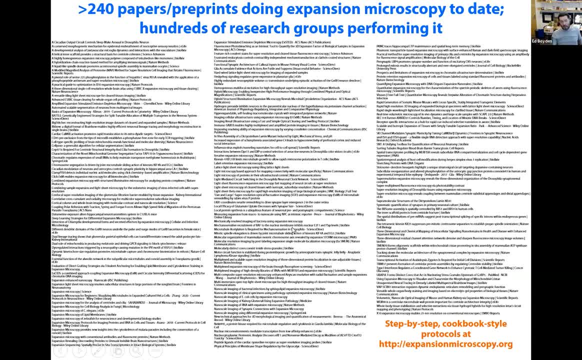 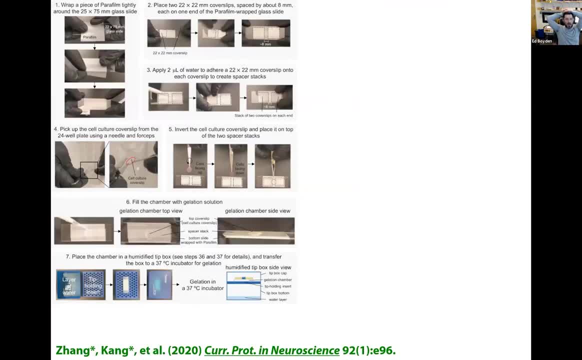 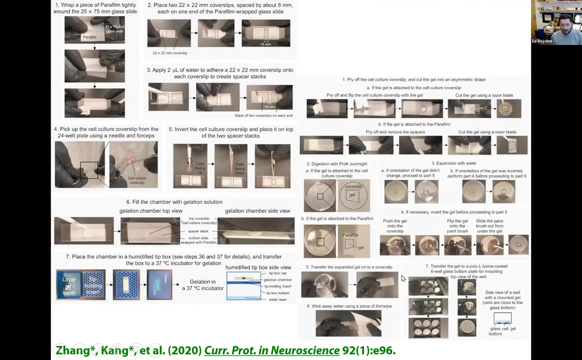 So the Чтобы method, which results in about the reaction time from bio bumblebees to microorganisms carry around very much similar pattern, not that AuRp fucking pretty but leaves quite a tiny image in the background. But I think it's an excellent reason we built this tool and we really know we need. 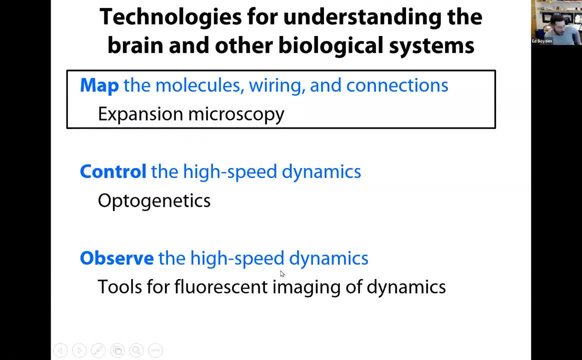 the economic capacity to do it. We know we can do it, So we're really seeing a change. so that concludes the first half of the talk. um and uh. yeah, if you want to give it a try. uh, really enables anybody to do nano imaging, so keep us posted. and the last half of the talk i want to 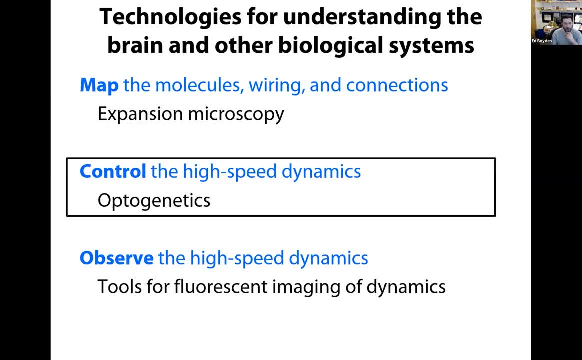 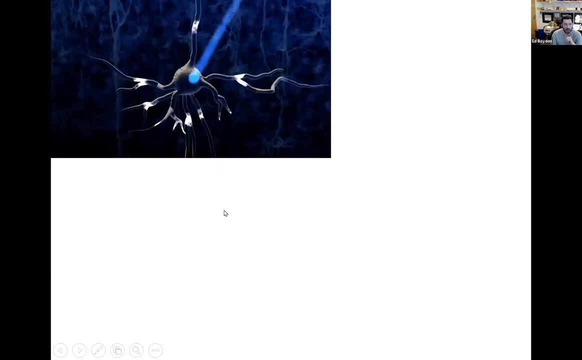 switch gears and talk about live signaling, control and imaging. i just want to have a few slides in optogenetics, because it's a fairly mature technology, um. so in optogenetics, opto for light and genetics. uh, because the reagents we use are genetically encoded. um, we take genes from the. 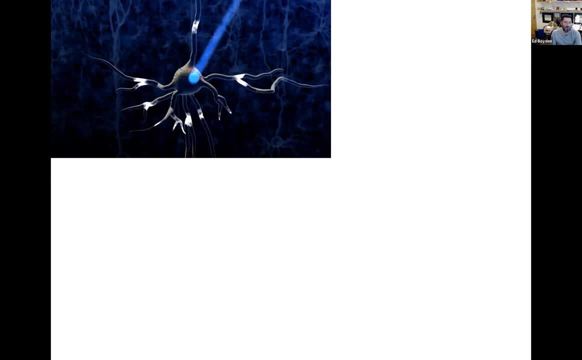 natural world and put them into brain cells. the gene products then make those brain cells controllable by light, and so this started when carl deisroth i were both students at stanford and we started brainstorming what are all the ways we could control neurons. and we just started. 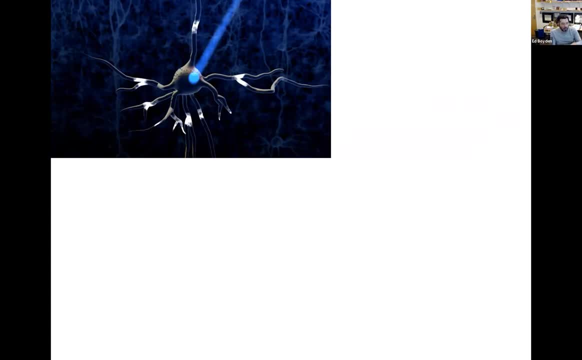 making a list of all the laws of physics. there's only so many kinds of energy you can deliver into the brain and we decided light would be the best if you could get away with it, because it's very precise and of course it's not going to be the same as light, but it's going to be the same as. 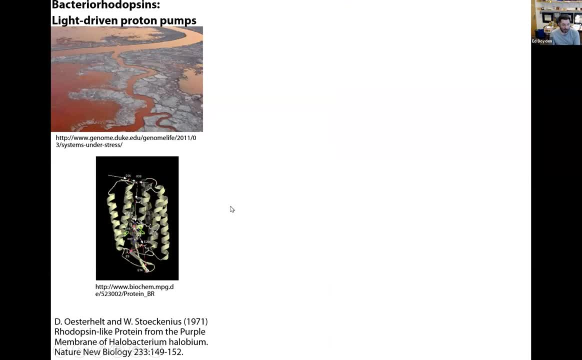 light, and we decided light would be the best if you could get away with it, because it's very precise and, of course, as fast as anything ever gets um. the next question was: do we make or find the light sensors? and i became really fascinated by this class of molecule known as microbial opsins. seven 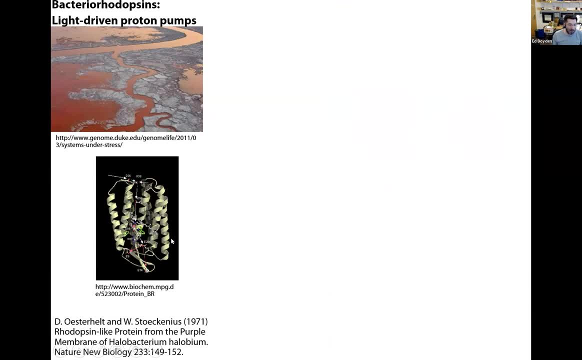 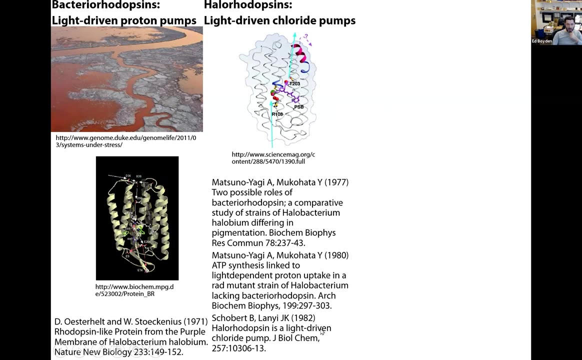 transmembrane proteins that sit in microbial membranes. a crystal structure of one is shown in the lower left. they're found in, for example, organisms that live in salty water. the first to be found was a light-driven proton pump about a half century ago, and then around uh, the early 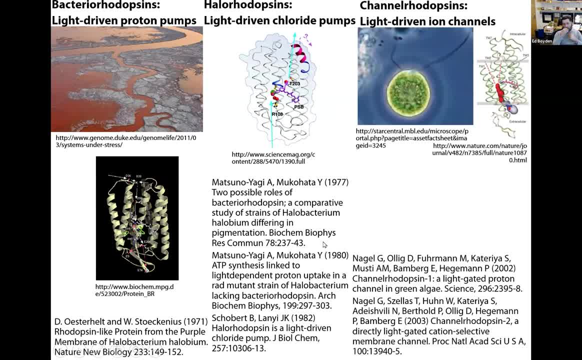 1980s, people found light-driven chloride pumps and then, around the turn of the millennium, people found light-driven ion channels. i'd make a long story short because much of this has been published some time ago. we found that members of all three of these classes of molecule 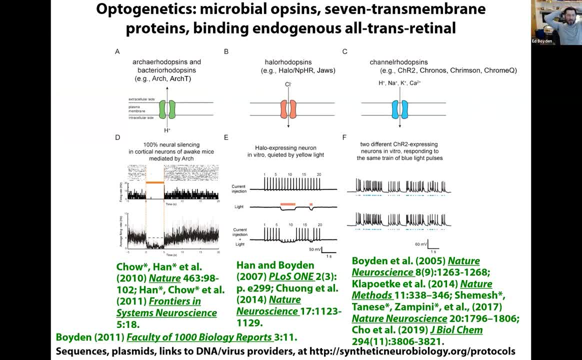 can be found that are fast enough, strong enough, safe enough and efficacious enough to mediate the optical control of neural activity. so light-driven proton pumps could be found that were safe, fast and effective in neurons. express the gene in a neuron with a virus, shine green or yellow light and you can turn those neurons off, work done by brian chow and. 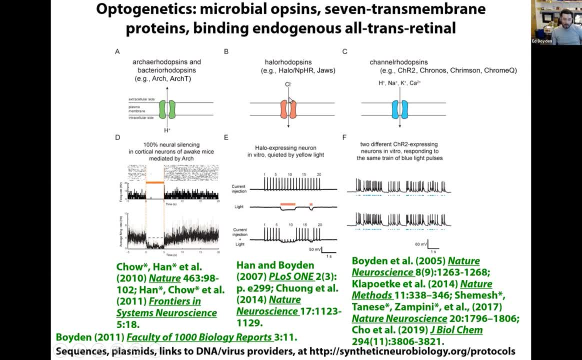 xue han when they work with me. light driven chloride pumps can also be found that are safe, fast and effective, and you can shine yellow or even red light to turn off neurons- work done by xue and also amy chuang. and then, finally, light driven ion channels can be found that are safe. 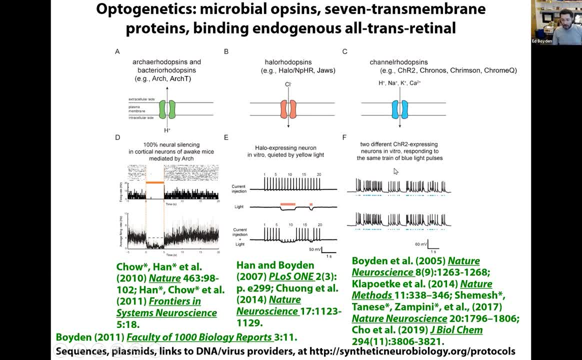 fast and effective. the first of these, carl and i put into neurons um and found that blue light could then be used to activate the neurons, and later nathan kopecky pushed this into the red and um orshamesh. collaboration with um, valentina miliani's group and others worked to 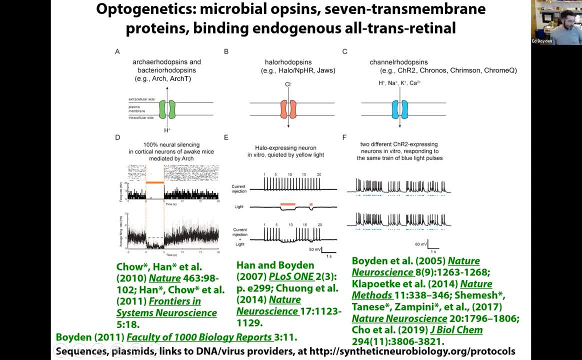 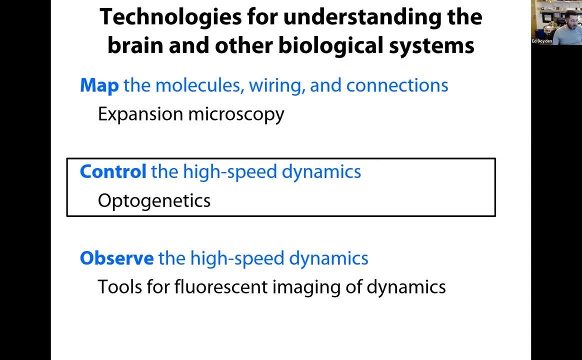 try to push these to their physical limits, and so these tools are in very widespread use to activate and silence neural activity. by turning neurons off, you can figure out what they're needed for, and by turning neurons on you can try to probe their sufficiency. i think that's all i want to say. 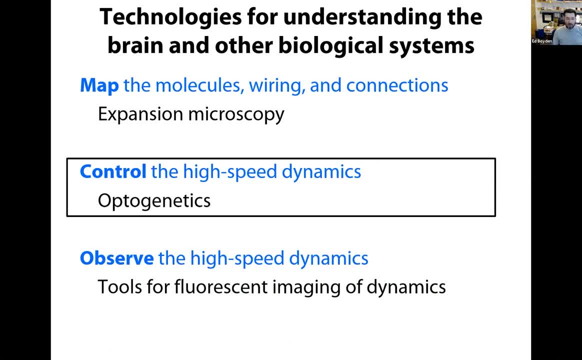 about optogenetics, because it is so mature and widespread, and i want to tell you about some new things that we're doing, um, which are the first thing we're going to do, is we're going to go into really, I think, exemplify this idea that we kind of lucked out with optogenetics and we have not. 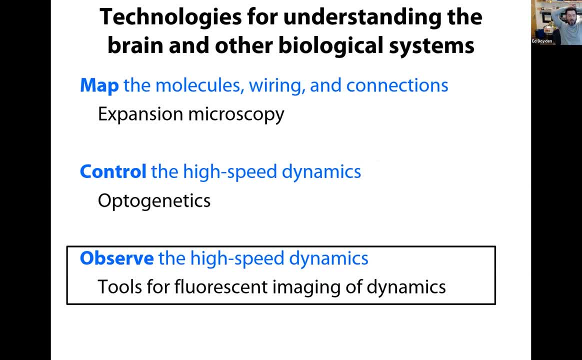 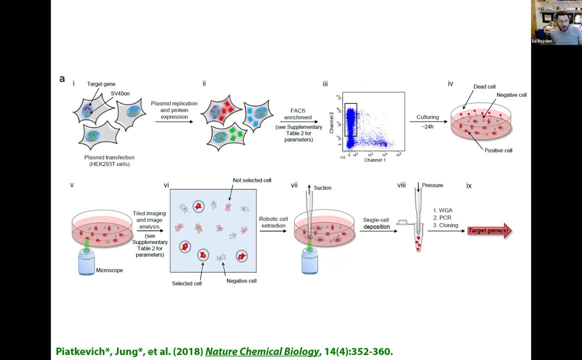 been so lucky for the opposite of optogenetics, which is: can we observe high-speed signals in brain cells? The natural world evolved optogenetic molecules that basically out of the box worked, but the opposite is not true. We had to evolve in the lab indicators of fluorescent signals. 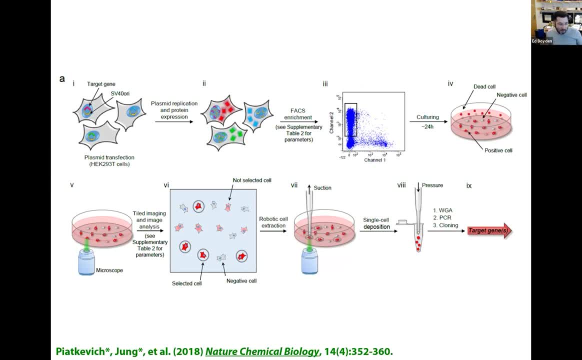 and we're not the first to do that, but we wanted to have a good way of doing it in mammalian cells. When Erika Jung and Kira Piakovich, our postdocs, worked with me, we wanted to have a way to take a. 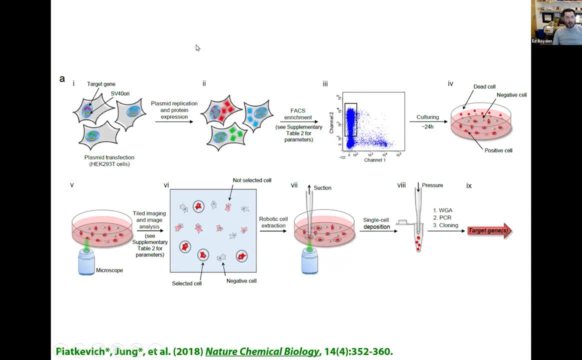 gene, make many mutants of it- some are better and some are worse- for any given goal and to screen the gene products on multiple dimensions- things like safety, speed, efficacy, the same kind of things that made optogenetics popular. We bring in a robotic arm and we can pull out the cells. 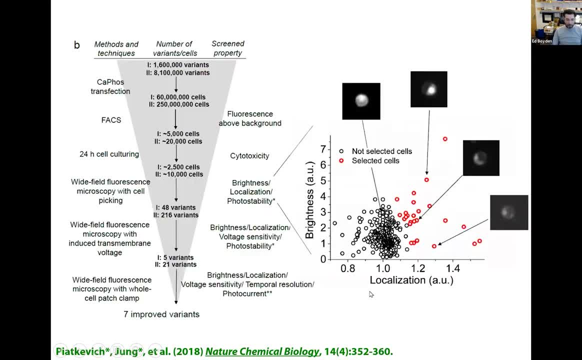 and therefore the mutants that are better for our goal. So we decided to first try to make a fluorescent voltage indicator. We started with quasar 2. From Adam Cohen's group at Harvard and in two rounds of directed evolution made 10 million. 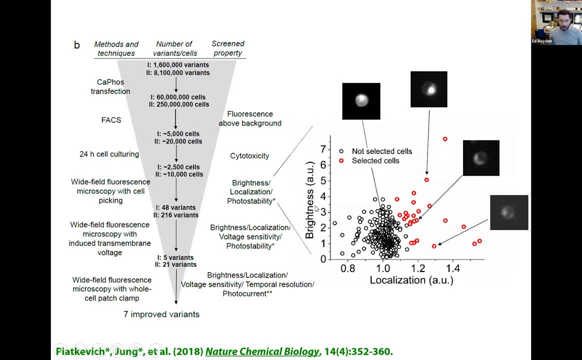 mutants, expressed them in cultured mammalian cells and selected in a multi-dimensional way for better brightness, better localization of the membrane and better photostability. I'll take the long story short. It's kind of a crowded slide, but in the upper left. 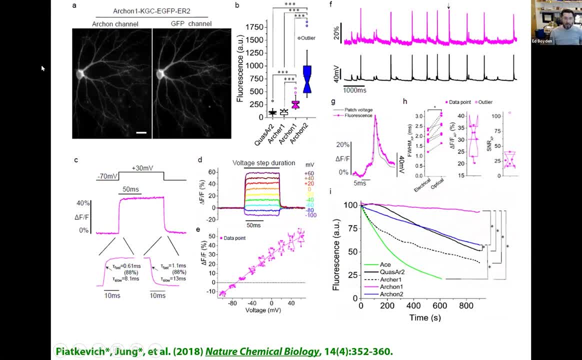 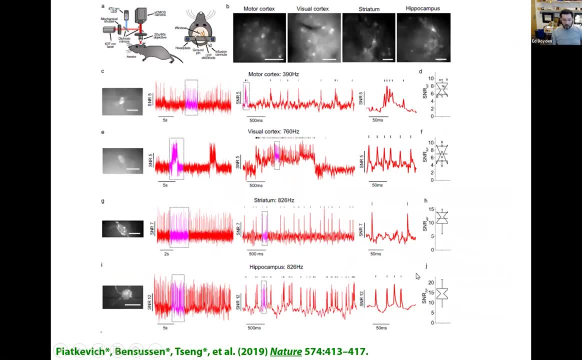 we made a molecule that we call Archon, which is better localized to the membrane than the parent gene. It has good signal-to-noise, as shown in the upper right, and it's pretty photostable. Working with Xue Han's group at BU, we showed that we could take a soma-localized version of 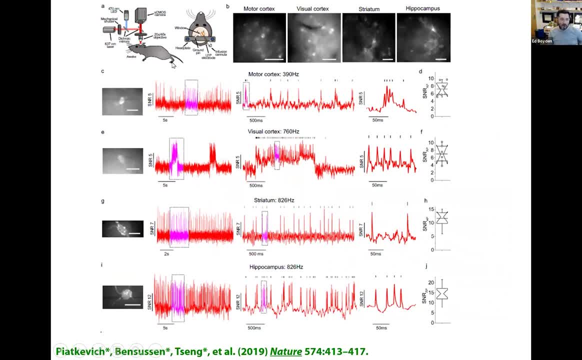 this to kind of clean up background fluorescence and, under a simple one-photon microscope, shine a red laser and collect the infrared light. you could monitor the voltage of neurons in awake behaving mice And even you could look at a population of neurons. Here are 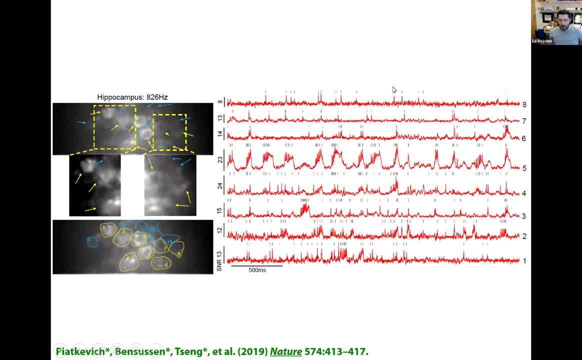 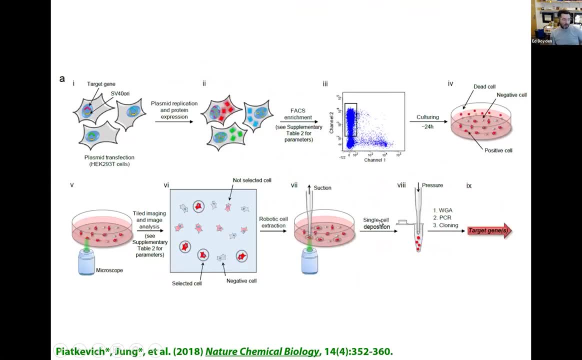 about a dozen neurons in the mouse, hippocampus, head fixed but awake, and on the right you can see about eight of those neurons were active during this movie And so this is very exciting. Can we use such a robotic strategy to improve all sorts of 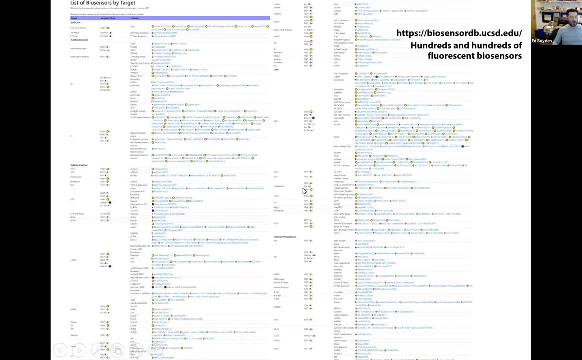 fluorescent indicators. Now, of course, we're not the first to make fluorescent indicators. This is a screenshot from Jin Zhang's database at UCSD where she has listed hundreds of fluorescent indicators- many from her group- that will light up when a cell experiences some change in calcium. 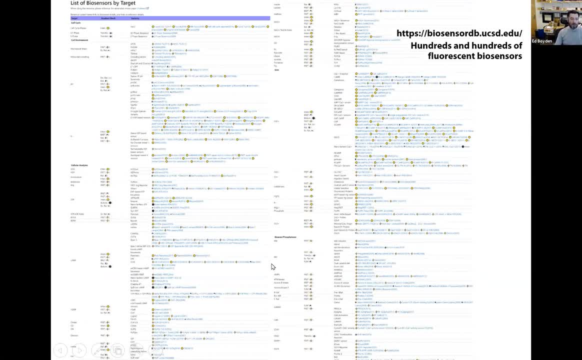 or cyclic AMP, or protein kinase A, And of course there are countless signals we'd love to look at. Wouldn't it be great to look at many signals at once? Cells take in inputs. They have such complex networks of biomolecules within. 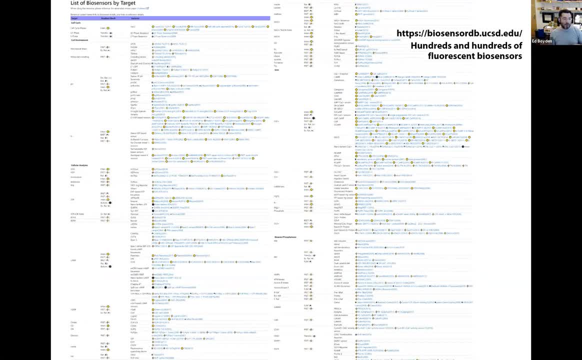 and then cells generate outputs. Couldn't we look at all of them at once in their interaction? Well, the classical answer was: make a couple indicators of different colors and you could use them together in the same cell, But that means you need to make a new indicator. 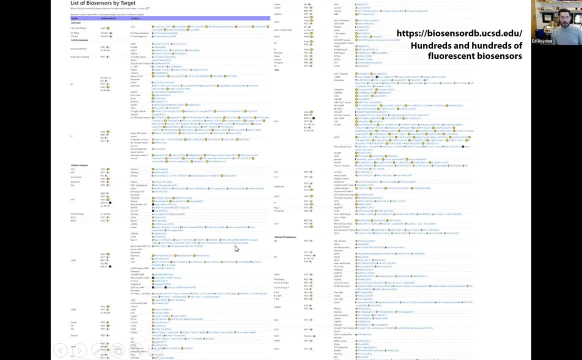 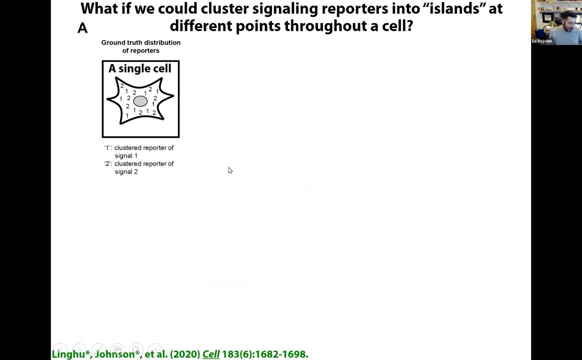 if you don't have one already, Wouldn't it be great to use existing indicators? Well, Shannon Johnson and Chengyang Linggu in our group worked on an alternative idea. What if we could park different fluorescent indicators at different points in a cell? Let's say the points labeled 1? 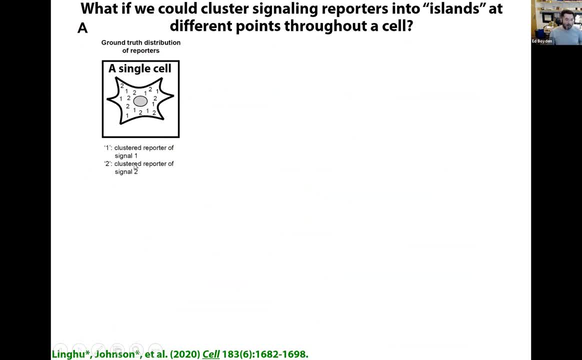 would have signal 1 being broadcast from those points, and the points labeled 2 would broadcast signal 2.. While the cell is alive, each dot will broadcast that signal, even if they're all the same color, and you collect little movies of the signals fluctuating. 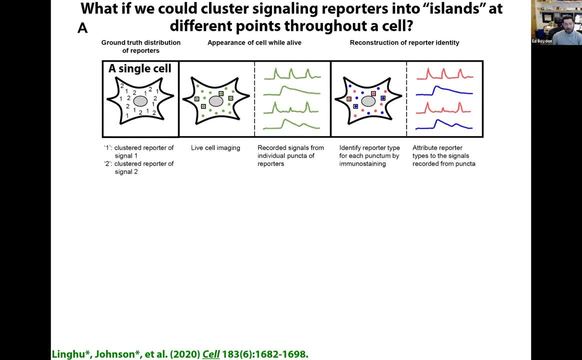 When you're done, you can stain, perhaps using techniques like I described in the first half of the talk. you can stain those dots with different tags and figure out which signals were at each point. Here's a protein architecture that makes it happen. 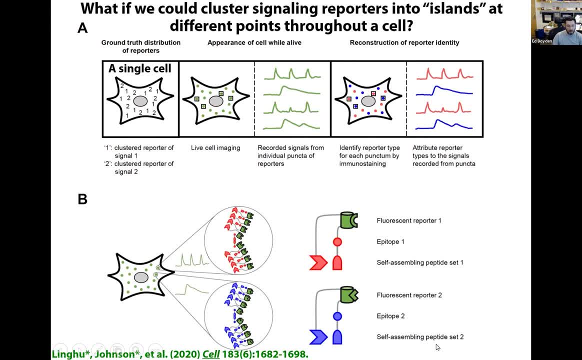 You can take different fluorescent reporters, infuse them to different self-assembling peptides, then they'll cluster at different points in space And if each reporter has a different epitope, then that epitope can be stained with an antibody, maybe over many rounds, so that you can identify them later. 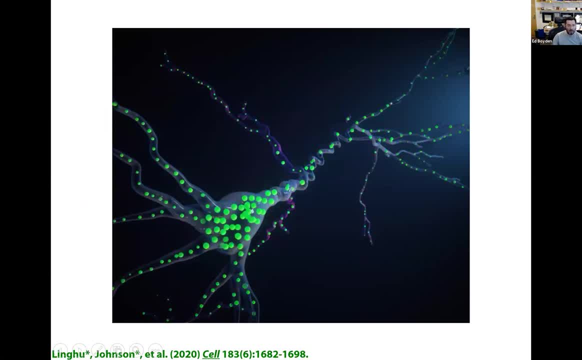 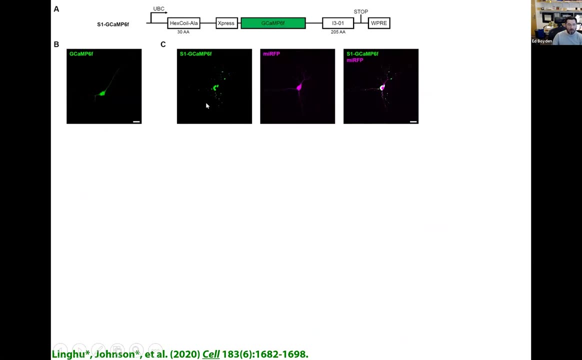 So here is a little cartoon. In green would be the live cell image In match. it would be the image of of the cell after you've stained it potentially over many rounds. And it works. So in panel B is GCaMP, a very popular calcium indicator. Panel C: we fuse it to a pair of self-assembling. 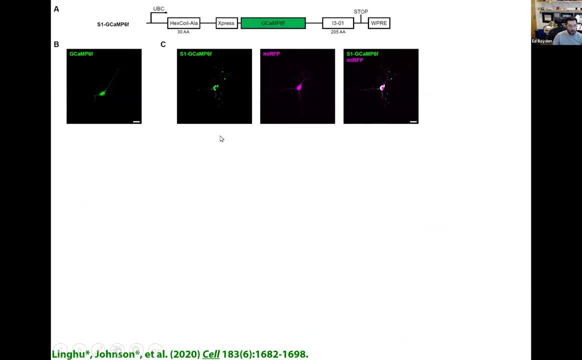 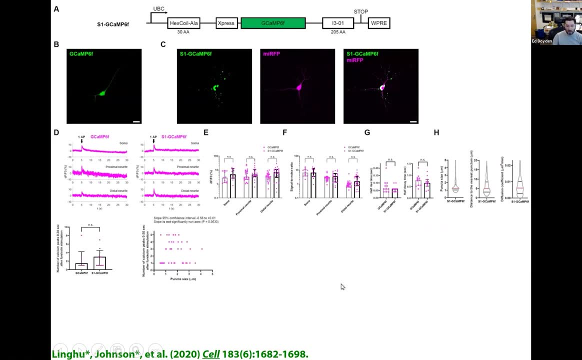 peptides. The pair seems to help it cluster better and it forms clusters. We did lots of control experiments, looking at signal quality, kinetics, endogenous physiology, cell health, synapse density, microglial reaction, you name it- And we didn't see any differences between. 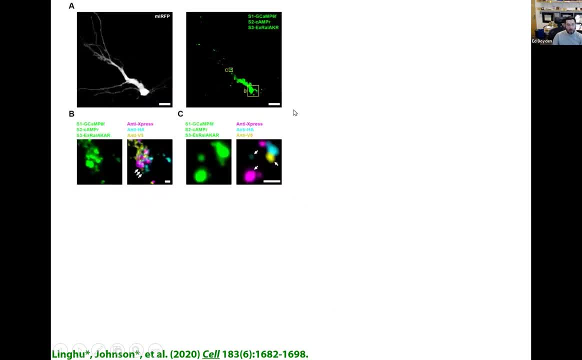 the clustered indicators and the regular ones. So now you can take three different indicators here for calcium, cyclic, AMP and PKA made by other groups. We fuse them to different self-assembling peptides, and epitopes In the green images are what you would see in the living. 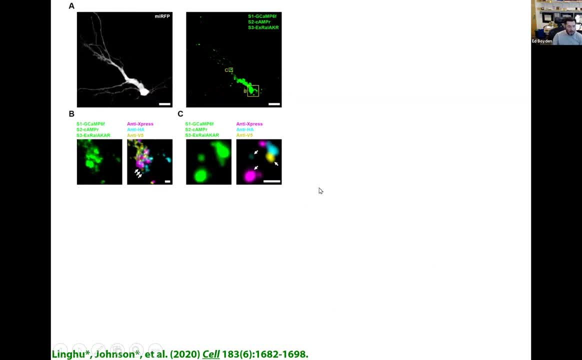 cell and the false color images are what you get after you stain with antibodies against the epitopes. So we can measure many signals at once in a living cell. This happens to be a cultured neuron and we can see the relationship between the different signals. In this case we're driving the cell with Forsklin and looking at calcium. 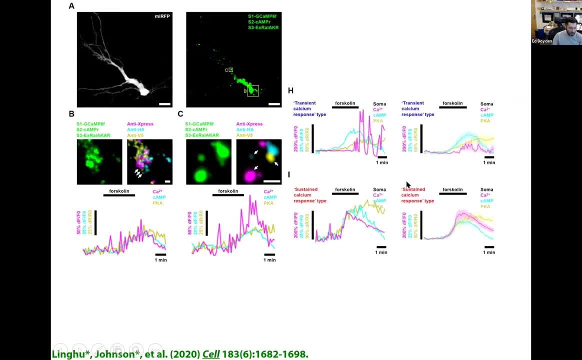 cyclic, AMP and PKA, and we can see relationships between these different signals, how they all relate to each other in time and amplitude. So we're very excited about this. Can we really parse out how all these different signals work out? Right now we're working to 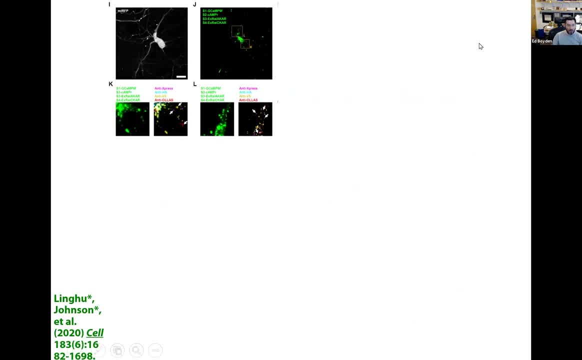 try to improve the technique. We've been able to get four signals at once to work in a single living neuron. Here we added a protein kinase C indicator. Again, green is the live and blue is the color image, and the false color image is when we stain. Here you can see four signals at once, or we 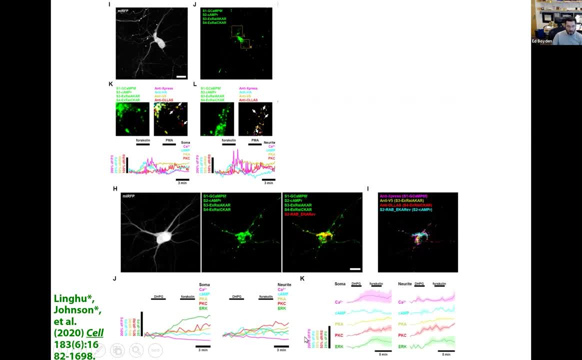 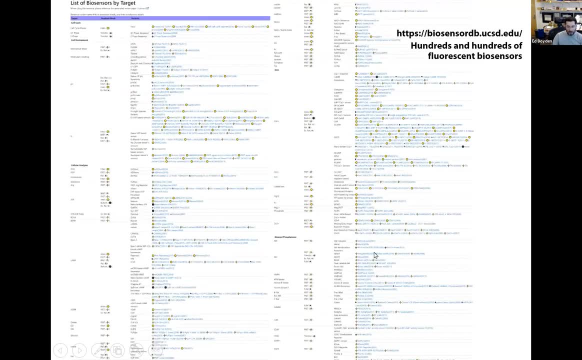 can even look at five signals at once. Here we added an ERK kinase indicator and you can see five signals at once. Anyway, there's a long way to go until we can look at everything. That's a long-term goal, But already I think there are questions that can be answered with the spatial multiplexing. 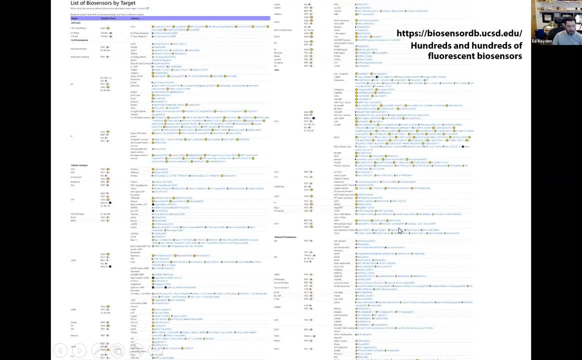 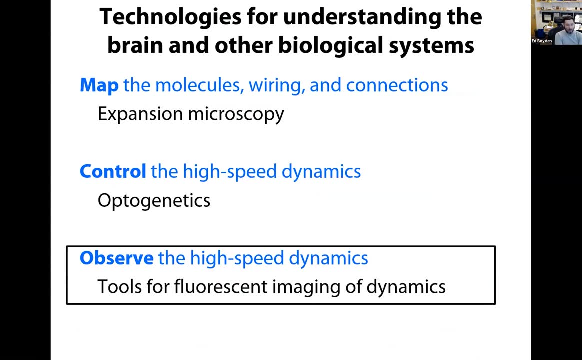 technology that are difficult to answer with older techniques. So to summarize the last half of the talk: yeah, with optogenetics we got very lucky. The natural world had evolved molecules that you know, out of the box we could use to control neural activity. But for imaging, neural and other 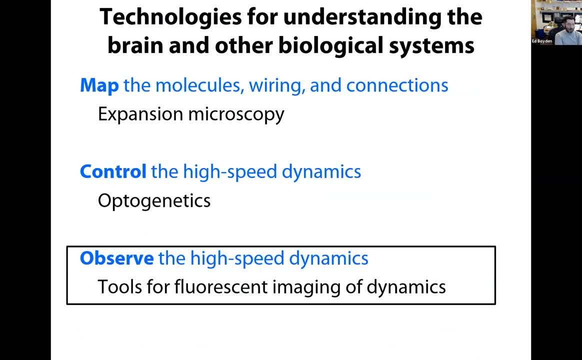 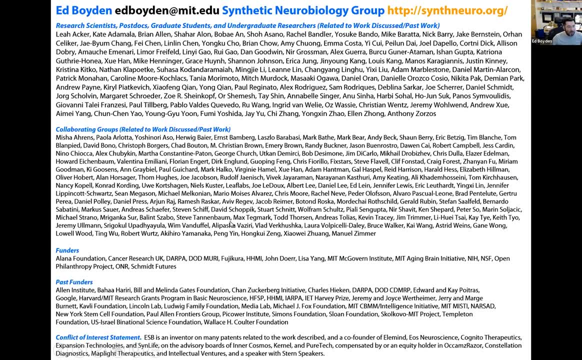 signals. we've been trying to both evolve better indicators as well as to figure out how to use existing indicators in new ways, And with that, I think, I'll end- Just to note that this, of course, is a very large-scale collaborative effort involving people all over the world. At the top, 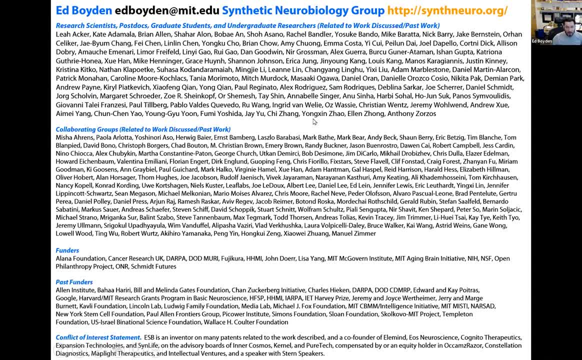 are people who helped with the projects in our group and our alumni. In the middle is an even longer list of people who helped with the projects in our group and our alumni. In the middle is an even longer list of collaborators who helped with the experiments that I talked about today.